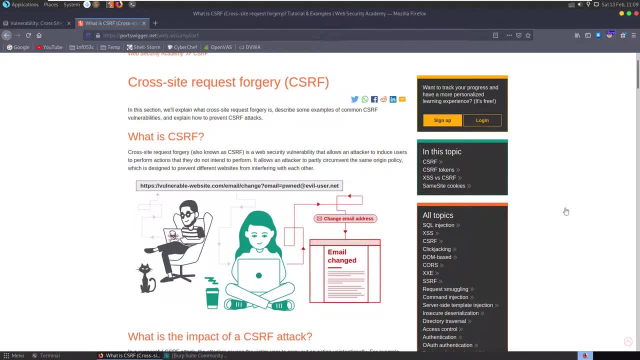 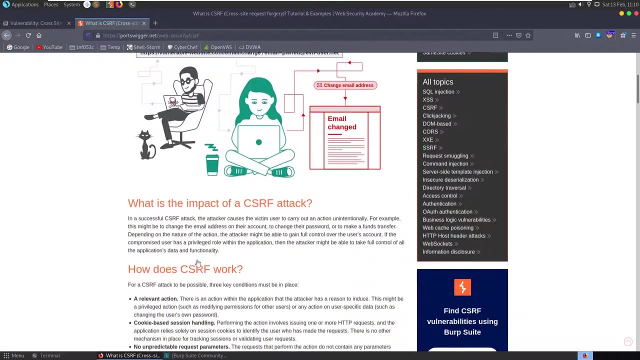 where they're already logged in using some cookies, and then it will automatically go and fill in the form or make the request to update the email address to the email of the attacker, so then the attacker could then go and log in, or maybe they'll change the password or something like that. So it tells us 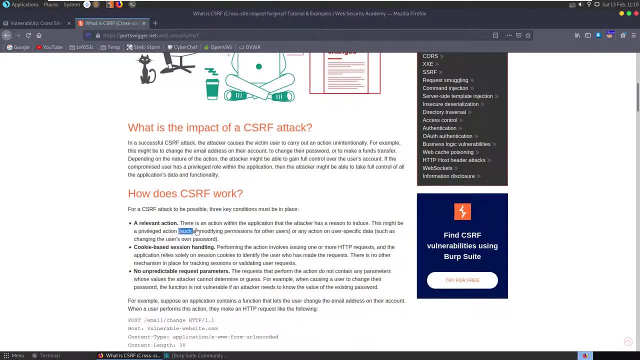 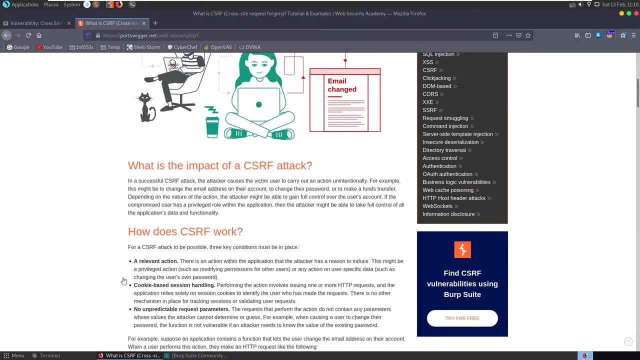 here that there are three conditions that must be in place for CSRF. so there must be a relevant action. there must be an action on the website that we're trying to get the victim to perform. that must exist on the on the site. There must be some cookie based session handling, so it needs to rely. 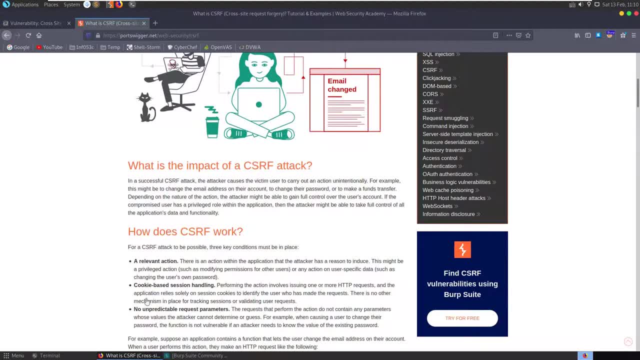 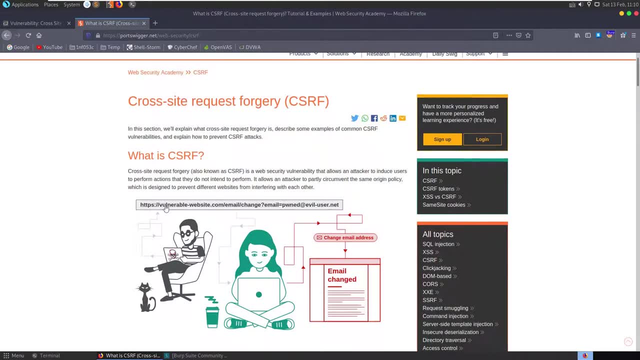 solely on session cookies to identify the user who's made the request. and then, finally, there should be no unpredictable request parameters. so we need to determine what parameters are going to put in here. so if there's a random token generated each time, that's not gonna work for us and that's the whole idea of. 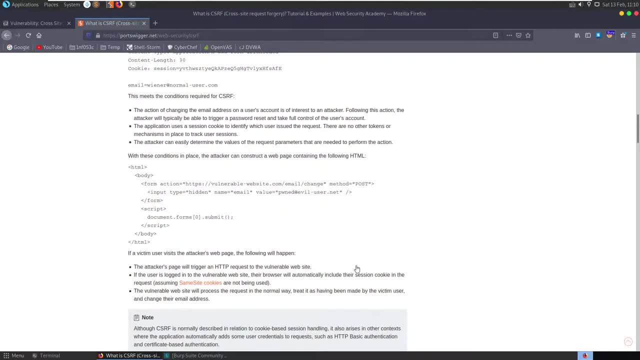 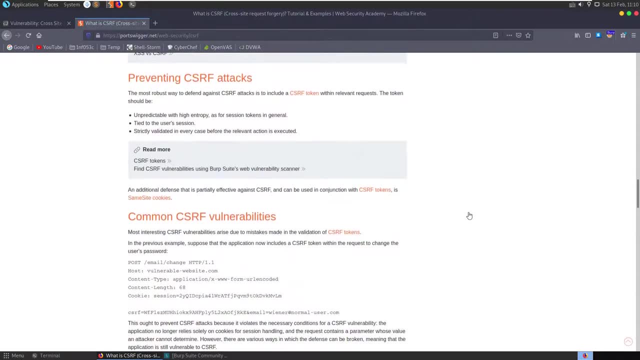 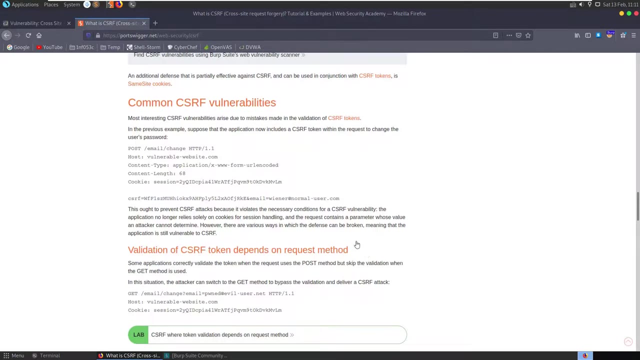 the CSRF token. so we in some of the challenges we've been through so far, if you think back to a brute force and challenge, we actually went through brute force in use and we would capture the CSRF token using the grep function in burp and then submit that with each each time we make the next request. we would. 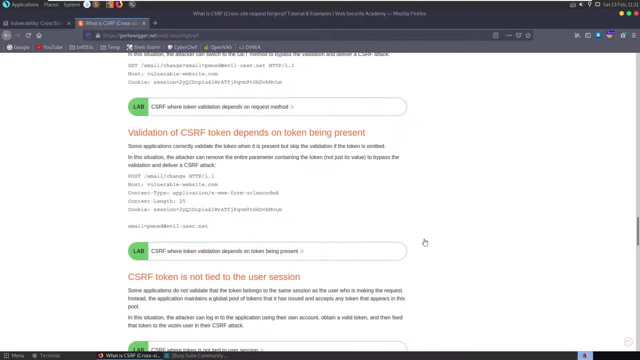 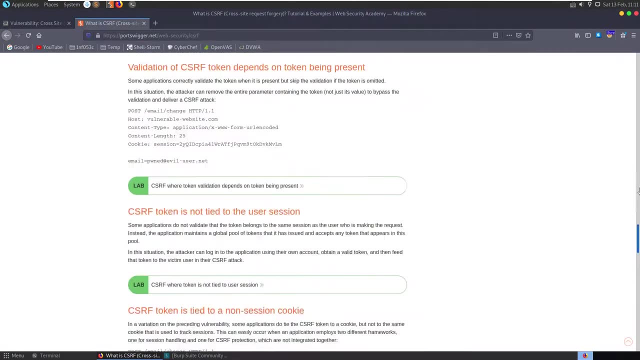 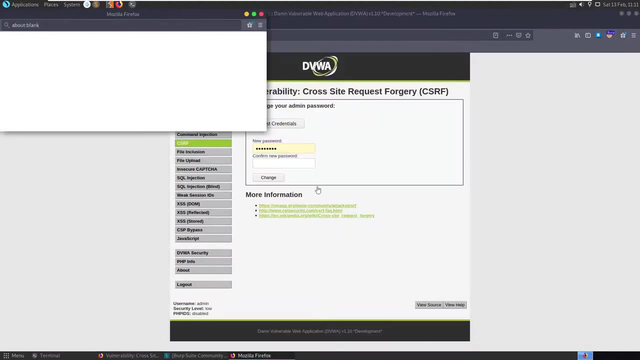 submit the new CSRF token. So there's some really good labs on here. you can see there's a lot of different labs and they get quite complex, so I'll try and come back and run through these at some point, but for now let's close that down. let's go back to our DVWA and check the help here. 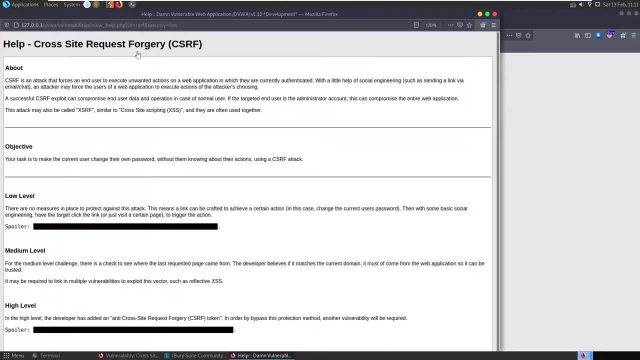 try and zoom in a bit. so same same thing here. CSRF, or CSRF, is an attack that forces an end user to execute unwanted actions on the web application they're currently authenticated with. with the help of little social engineering, such as sending a link via email or chat, the attacker may force the user the web. 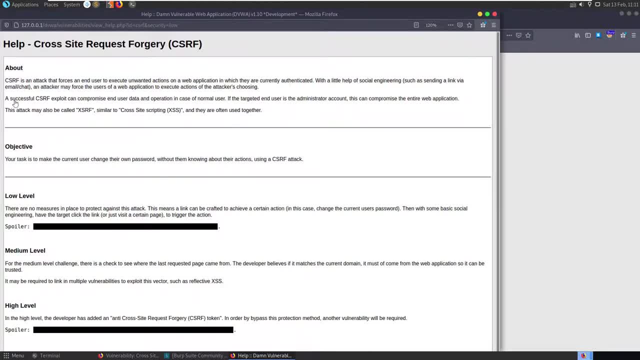 application to execute actions of the attackers choosing. It may also be called XSRF, similar to cross-site scripting and often used together, and it just mentions here that if the target end user is an admin, then it can compromise the entire web application. so let's see what our goal is here. the objective it 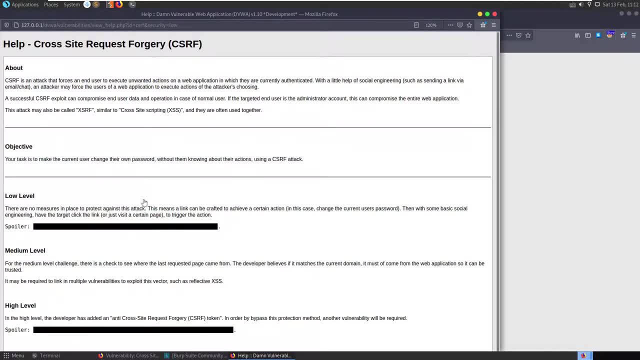 says is to make the current user change their own password without them knowing their actions, using a CSRF attack. and low level says there are no measures in place protecting a server from the cSRF attack. and low level says there are no measures in place protecting a server from the cSRF attack. 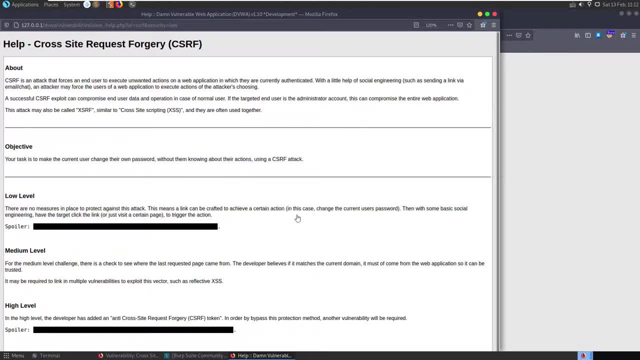 attack. this means that a link can be crafted to achieve a certain action. in this case, change the current users password. then, with some basic social engineering, have the target, click the link or visit the page to trigger the action. so let's close that down. let's try and see if we can do the low. 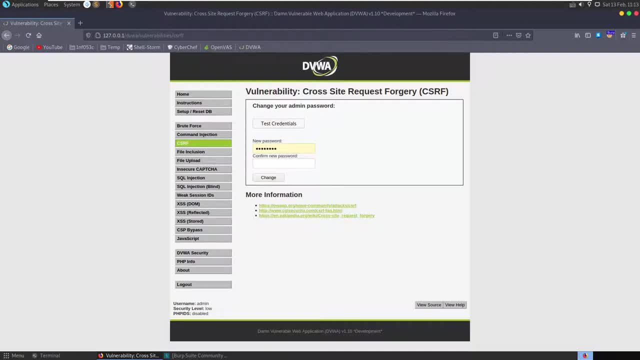 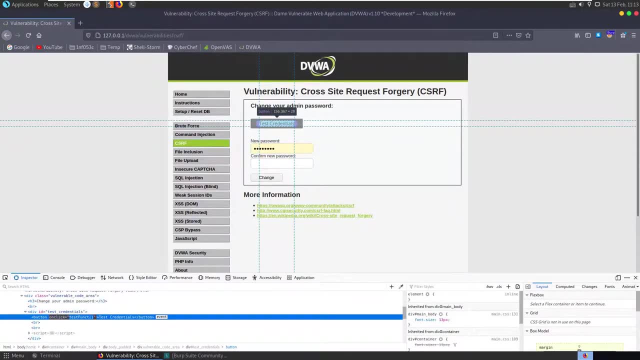 difficulty. so let's have a look at the form here. if you inspect this element, we have the test credentials function button on click test funk. okay, we have a script here where it's going to call window open vulnerability, CSRF, test credentials dot. PHP. okay, some of this might be to do with actually verifying. 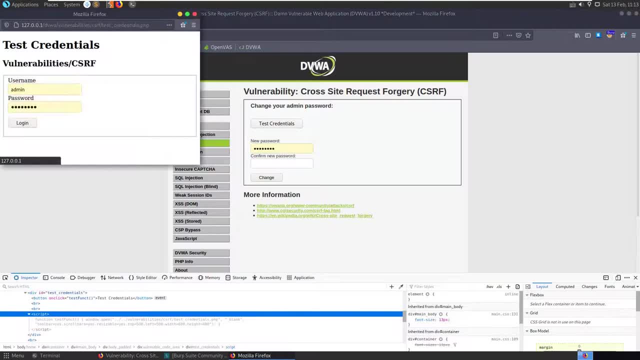 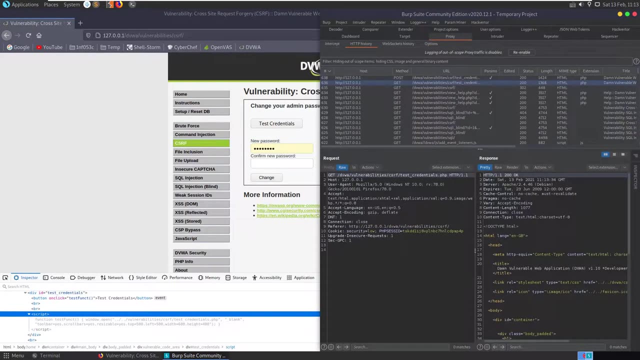 that we've done the challenge. let's let's hit test credentials. you can see here it's asking for username and a password. let's login: valid password for admin. okay, let's have a look at our burp suite. look at the requests. have this test credentials. so we make the get request first. we made the get request here and 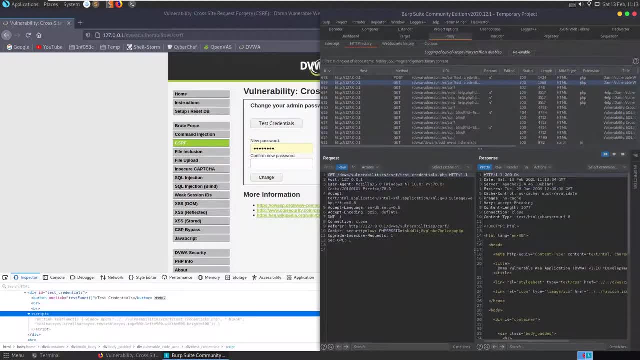 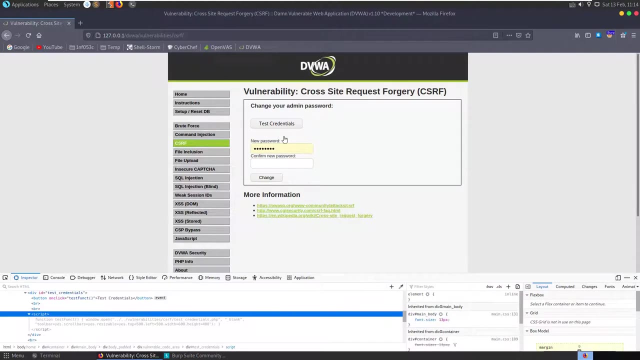 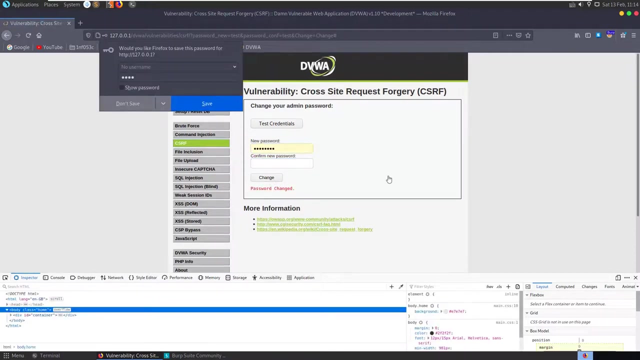 we redirected. it made the get request to the test credentials and then asks us for the username, the password, and then finally it made this post request where it sent our username and password. so let's looks like that's the valid. maybe let's try and enter a new password here, let's say test, test, change password. 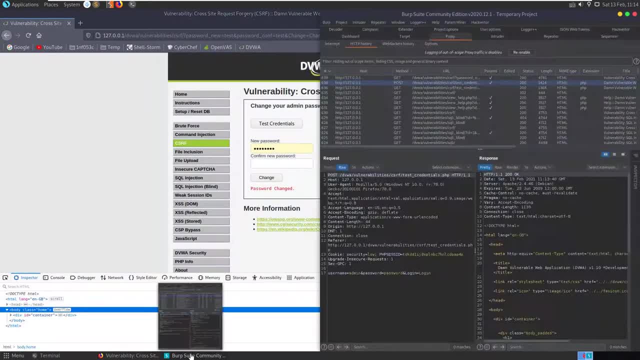 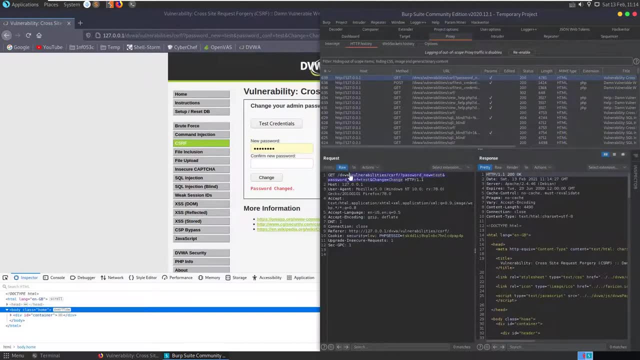 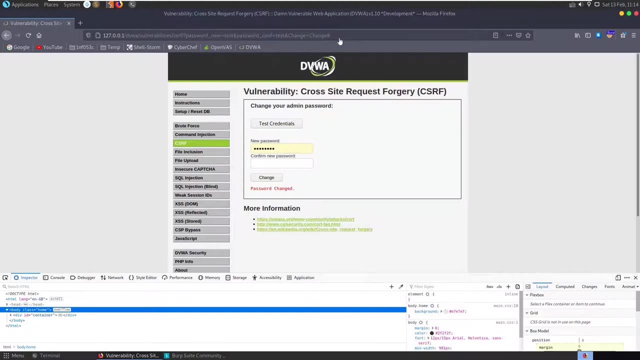 changed. okay, let's check out burp suite there and see what happened we got. we had a get request and the get request simply sent off. this password new is equal to test. password confirm: equal to test. okay, so if we were to take a copy of that and insert that, oh, insert that here and let's say: test one, two, three. 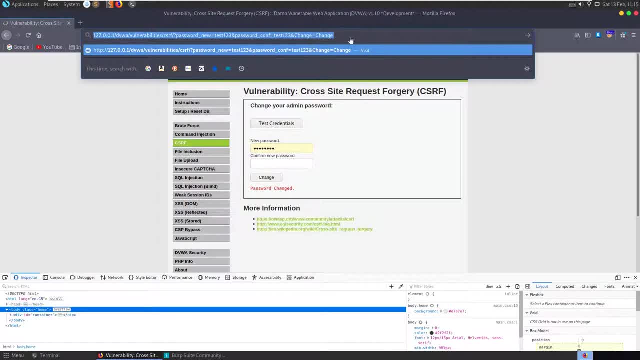 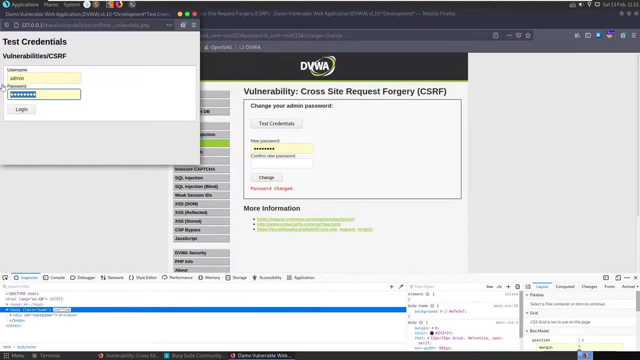 test one, two, three. copy that if we were to access that URL we'll get: the password has changed. let's test credentials and say admin and then test one, two, three. we can see that a valid password for admin. so let's go back and change our password here, because otherwise I'll forget what it is. it was just password. 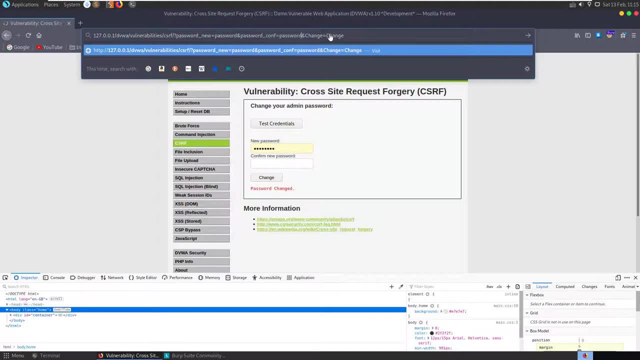 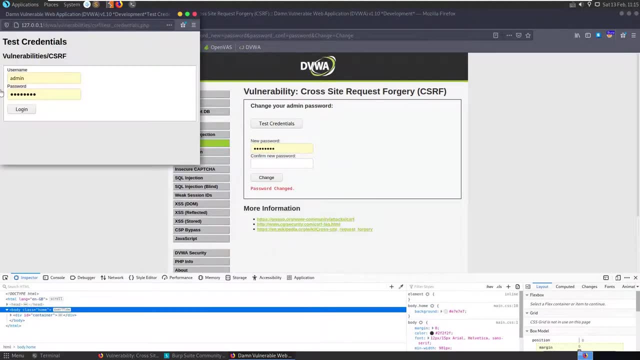 this is the password that we use to log into the application, by the way, so make sure you know what it is. so we save that. let's test it again, admin. this time it's gonna be with password and there we go: valid credential. so essentially that was. 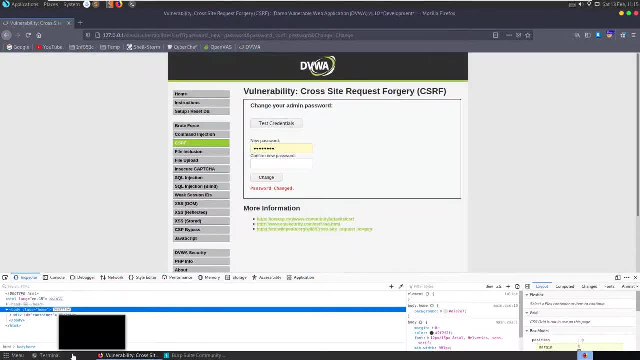 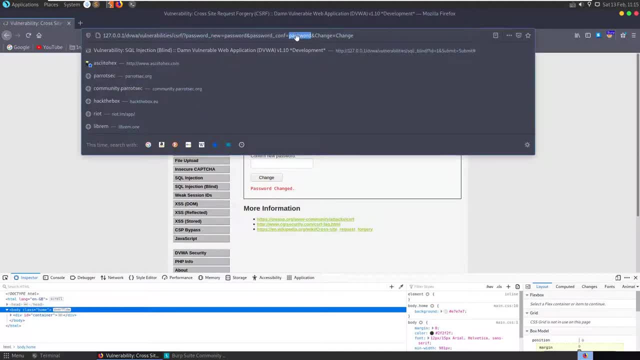 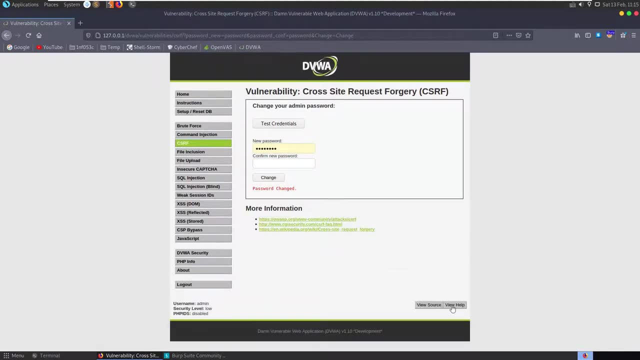 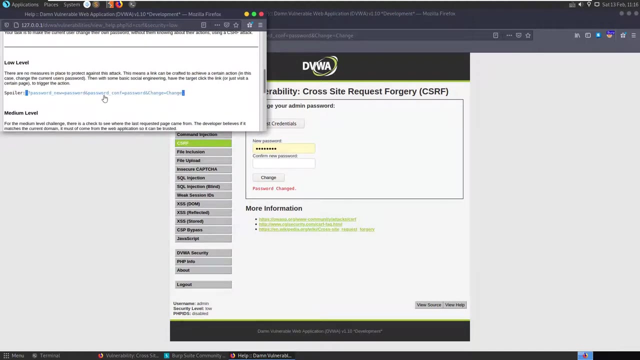 that link and it changes their password to our password of choice and then we go and just log into their user account and that's essentially that. let's take a look at the help and see if they suggested anything differently. okay, so it's just telling us, just giving us the URL, and let's check out the medium. 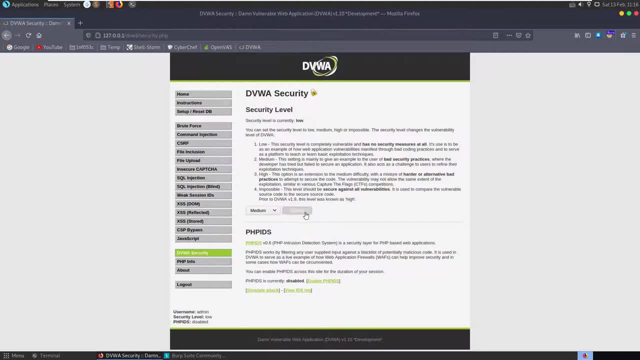 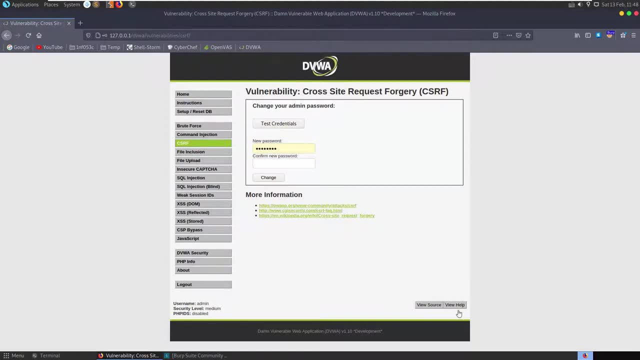 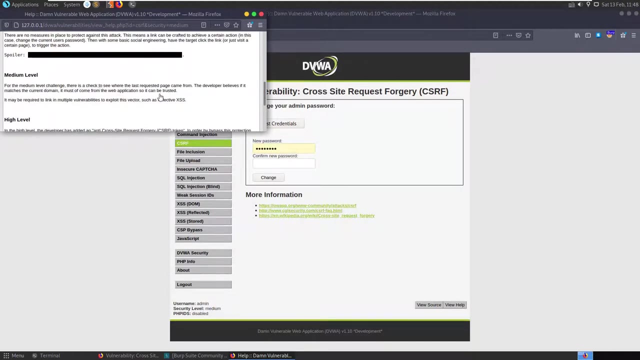 difficulty, then let's go and change the security level, change that to medium and submit and go back to CSRF. so for the medium difficulty here, if we check the help section it says medium level. for the medium challenge there's a check to see where the last requested 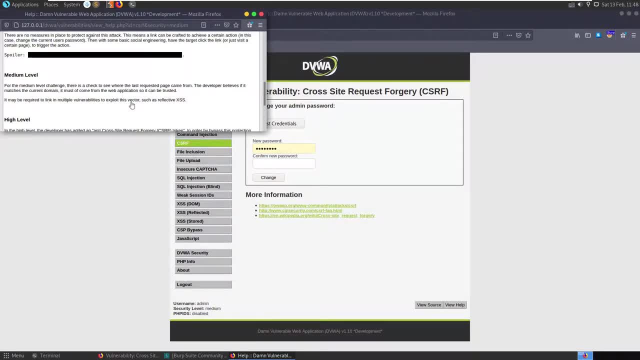 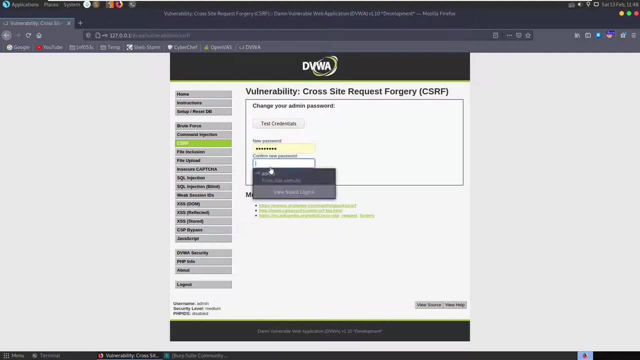 page came from. the developer believes it matches the current domain. it must come from the web application so it can be trusted. it may require link to link multiple vulnerabilities to exploit this vector, such as reflective XSS. so to give an example, let's change the password here. well, the password is already at. 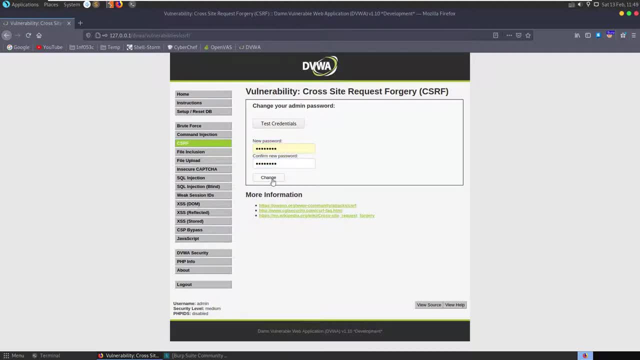 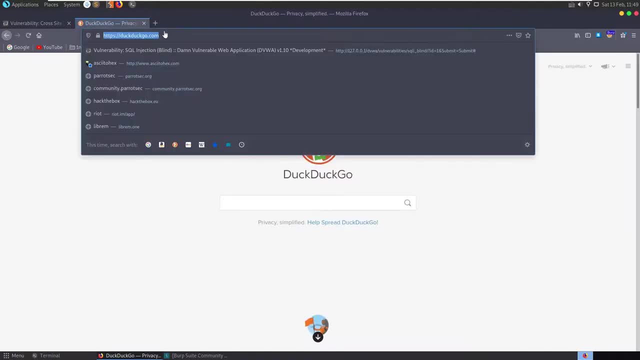 password. so let's just change it to password, hit change, just so we can get this URL. and what I want to do out of interest is just go to. let's go to our home page and then let's pretend that we're a victim. somebody's just sent us that URL and we're gonna access it to change the. 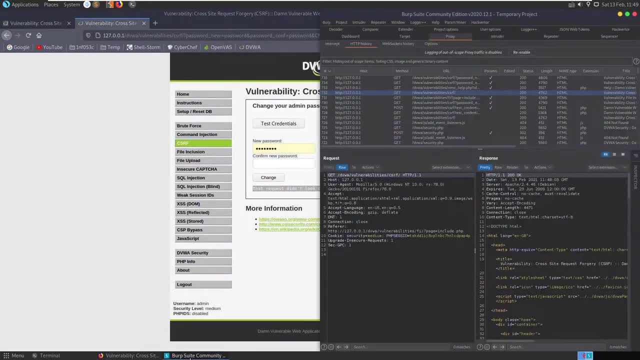 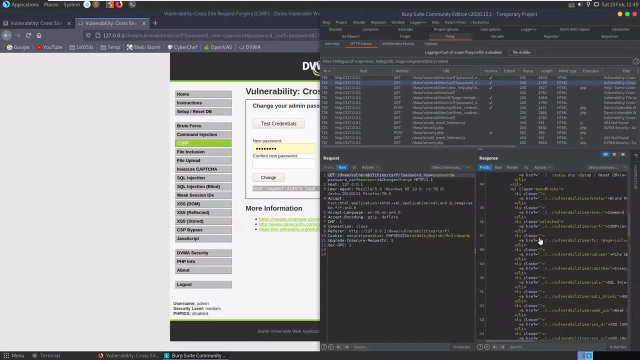 password. we hit that and we get that request didn't look correct. so let's take a look at the request. the first request that we sent you change the password. you can see here it came back, and this one successfully, whereas it's password changed, whereas this one- we got that request didn't look correct. 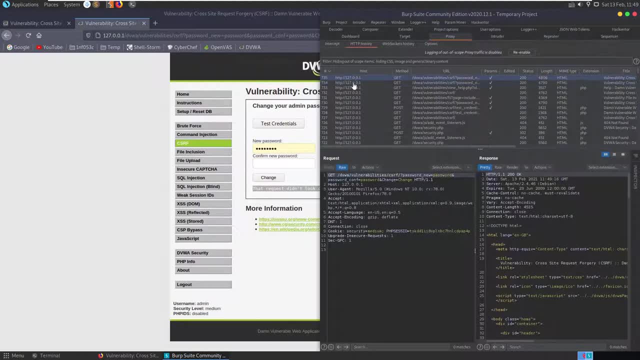 and if we look at the differences between the two requests, we can see straight away there's a header missing, which is the referrer header. so in the first one we had a referrer header to say we're coming from 127.0.0.1. the. 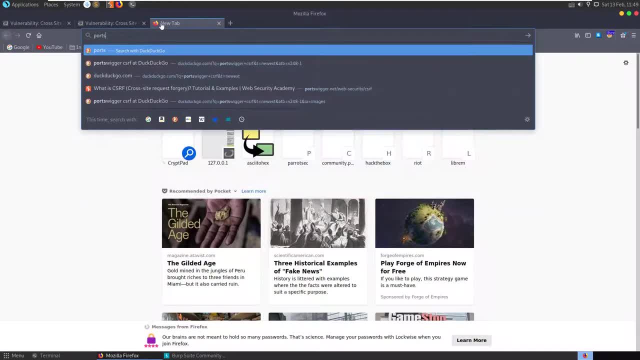 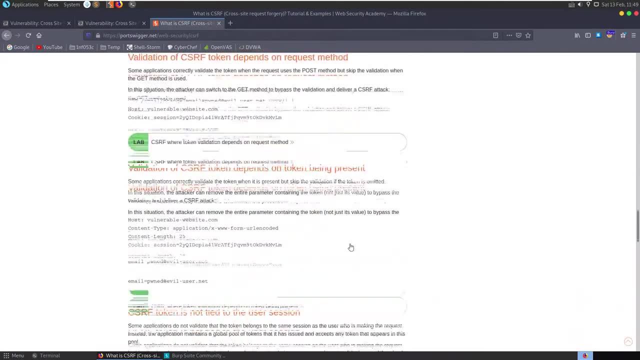 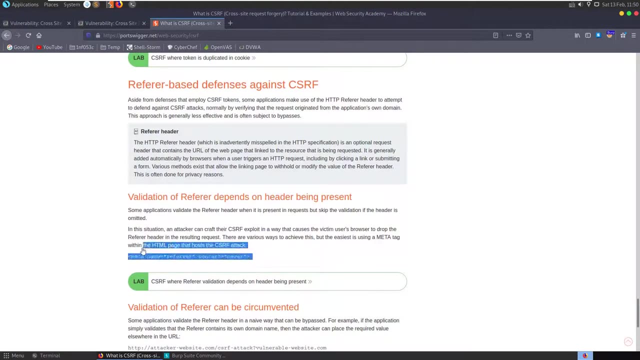 second. we didn't, so let's just remind ourselves. let's go back to the port swigger CSRF documentation. if we scroll right down to the bottom, there's a section here on the validation of referrer header. so in some cases removing the referrer header altogether might bypass the check. in other cases it suggests: 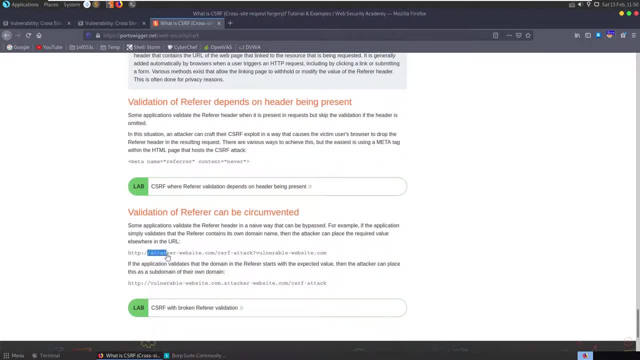 here that you could. if the. if the referrer header is checking to see if it contains vulnerable websitecom, you could potentially send a referrer header to your attacker websitecom but then have their URL at the end. just depends how the they're actually checking the referrer header. if they're simply. 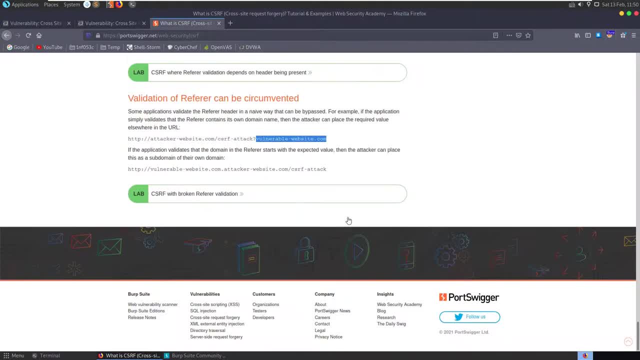 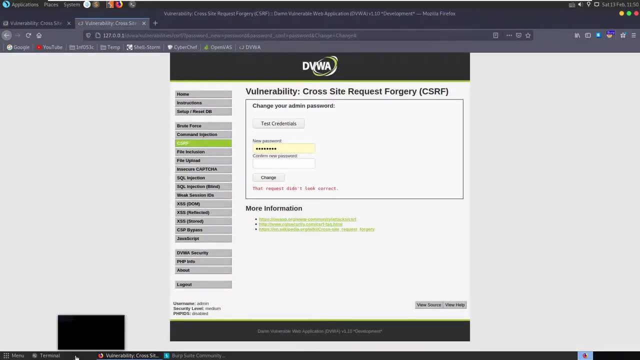 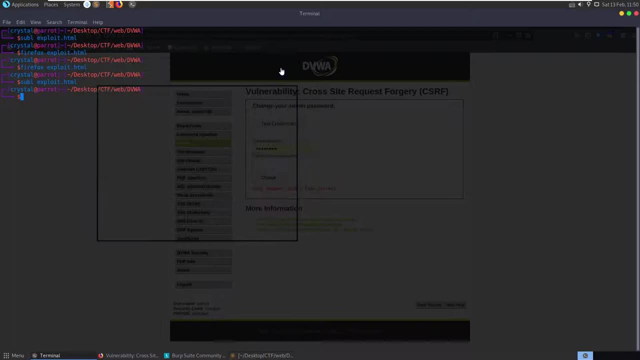 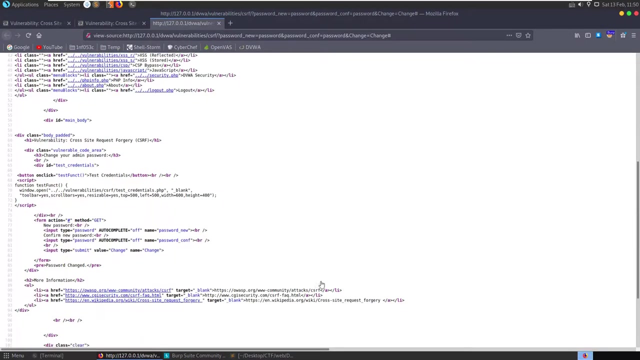 checking to see if the string exists within the referrer header and that attack might work, so worth bearing in mind in this case. inflating around with this, I was looking to create a form. here you can see, you create a form, exploit HTML, and essentially i took this from whereas it's. let's view the source. we can see. 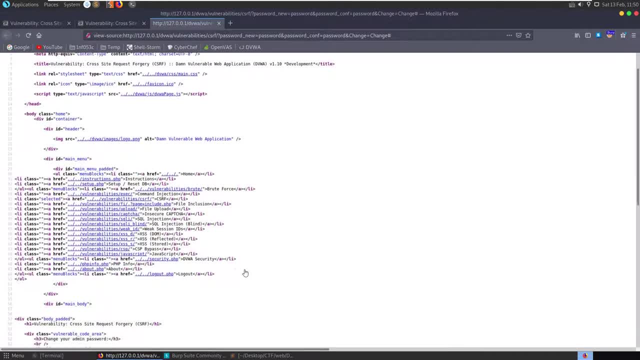 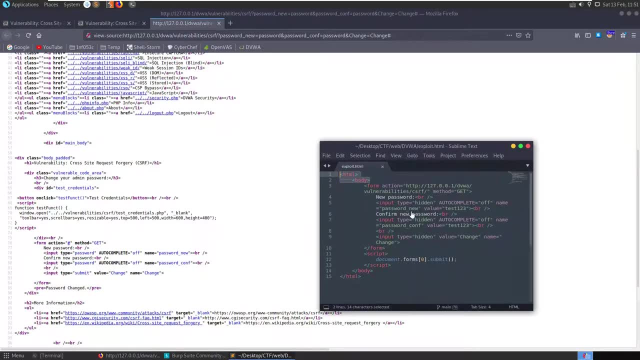 here that we have our forum to change the password. so i created a short HTML file and just in the body put in that same form. but we put in our actual URL and see here, instead of the hash because we're going to be sending, say, let's pretend that we're hosting this. 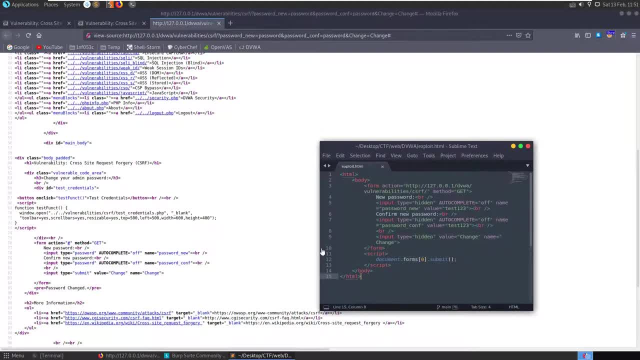 on our server and instead of it being dvwacom, it's going to be dvwocom or something, and we send them the link and it has this hidden form. so we've changed these fields to be hidden, so they won't actually see anything, and then, rather than just the name being set here, we've 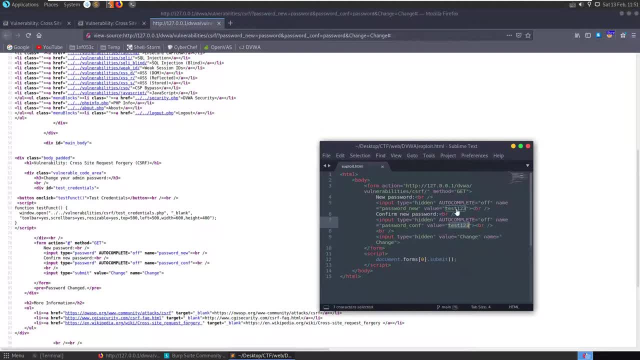 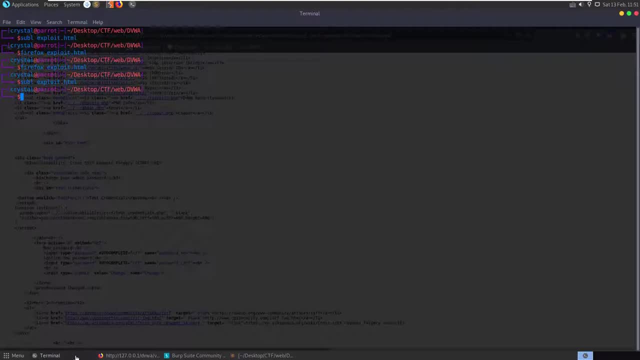 also set the value to say automatically, and this is the password we want to set, and then we have everything hidden. we just automatically send the form, and then the page should just close. so let's, let's open that firefox, firefox exploithtml. you can see it just instantly. 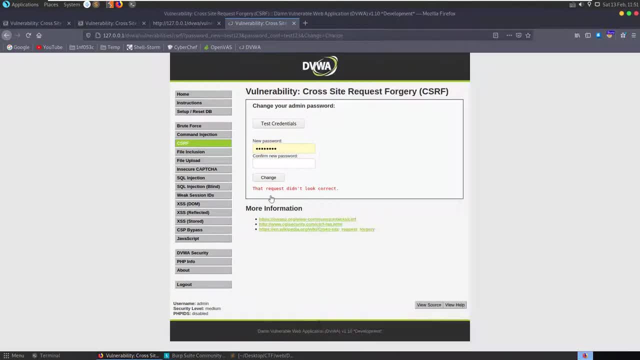 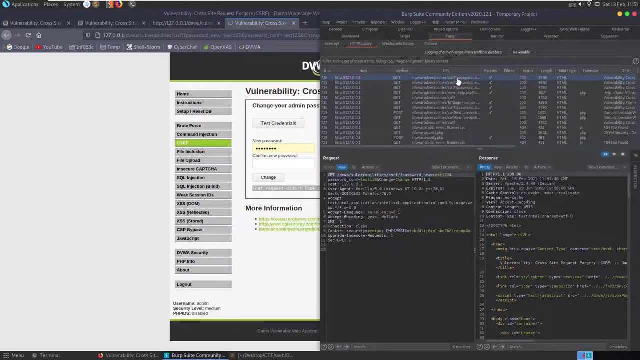 closes if we go to our. but we get this. that request didn't look correct, so it redirects us here. let's go to burp suite and we'll see that we got this request. and again, the issue is that we've got this request and we've got this request and we've got this request and 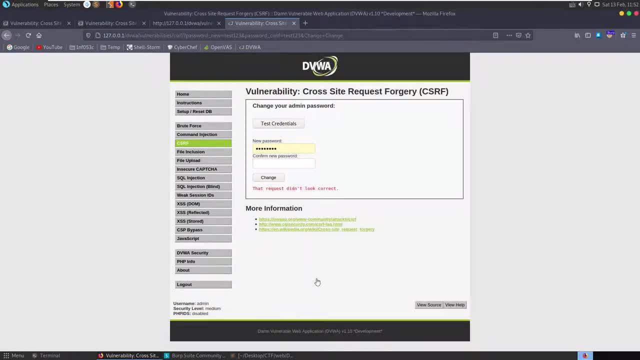 the issue is that it didn't have the referrer header here, so we've described one way that we could potentially bypass that. let's go to our stored. okay, actually, let me clear that we haven't gone through through the stored xss yet, as was working our way down, so i haven't actually done. 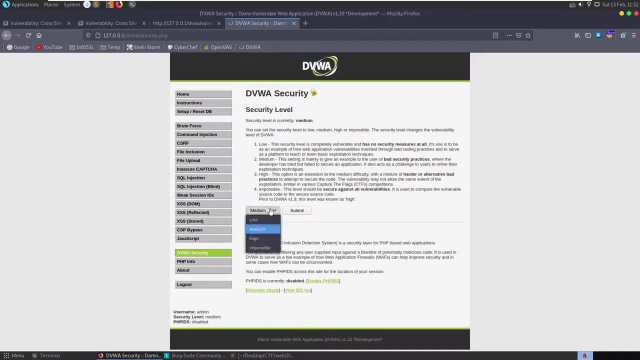 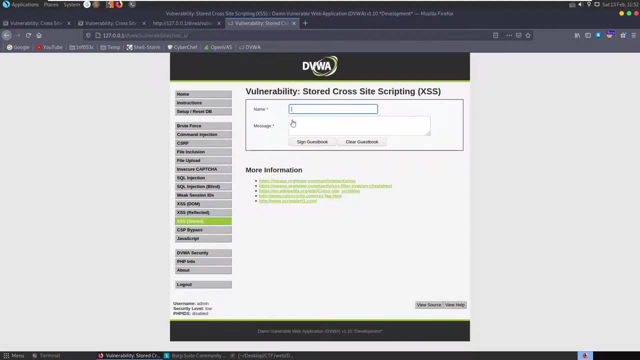 this yet, but, and what i'll do is just go and set the difficulty to low just while we store our xss, not worry about any protections that might be in place here, and we just want to say, um hi, admin, we have a message for you, and the message is going to be: take a look at this image, please, and the image contains: 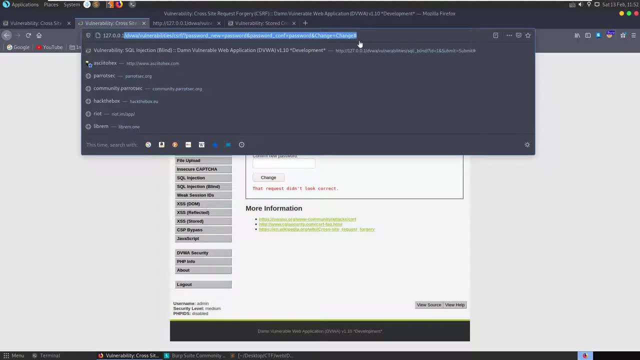 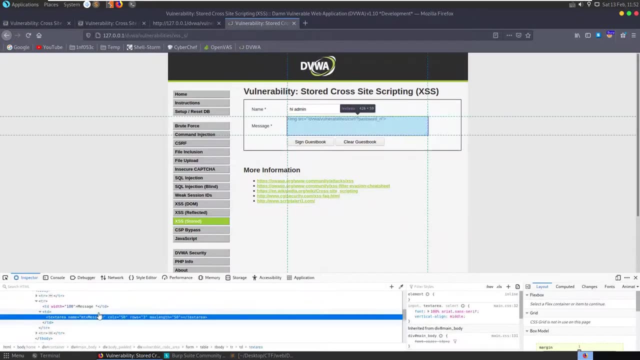 our url, so let's copy that. okay, we can't fit the url in. let's inspect element. set that the max length to 250 and let's just paste that in there again, you'll see there, we paste that in. let's change the password to test. 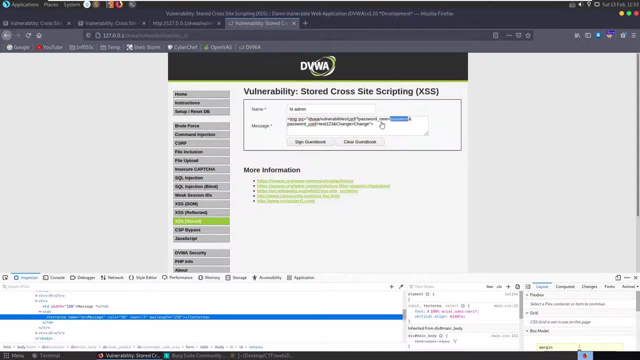 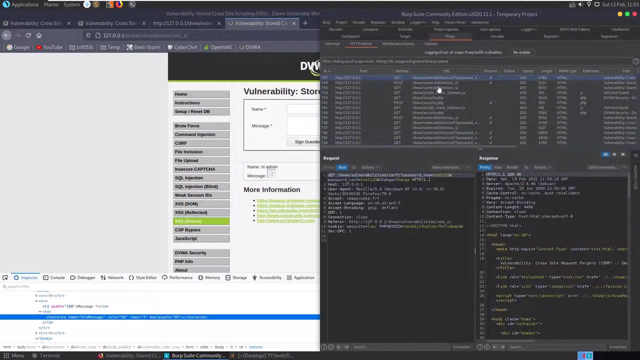 one, two, three and test one, two, three. sign the guest book. you can see here we've got a little funny image. because it didn't recognize that image, it actually interpreted it in code as code instead, and if we take a look at our burp suite, here we have a get request, so we have this post. 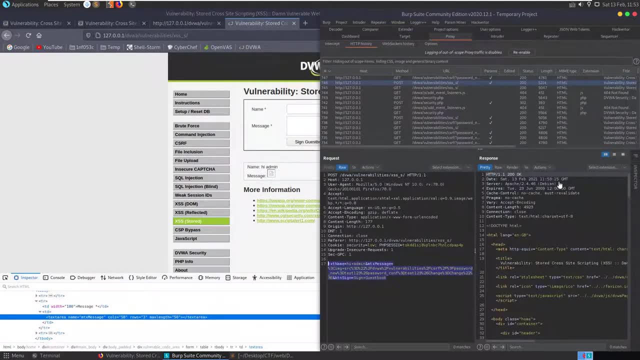 request here where we submitted to the guest book and then immediately after- let's see the timing on this- 15 seconds past, we have this at 16 seconds past. we have then a request to change the password and you can see that a referrer header is set from the xss screen that we were on. but as long as the 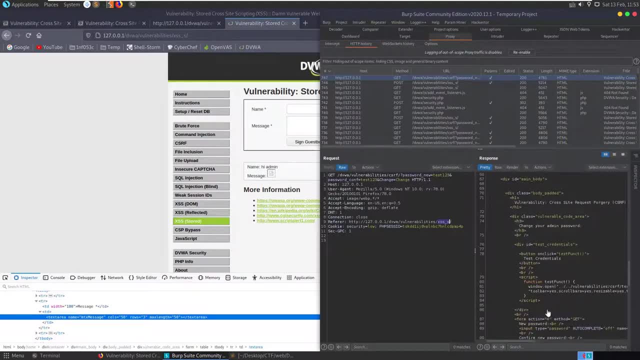 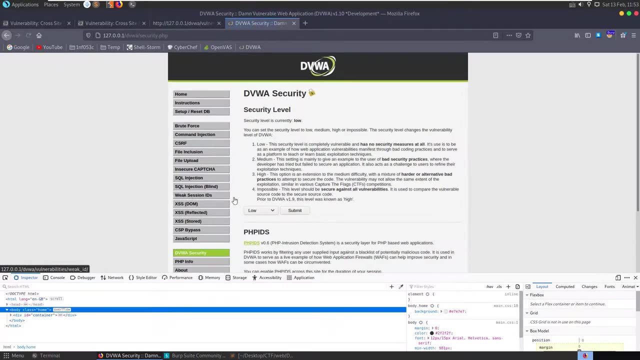 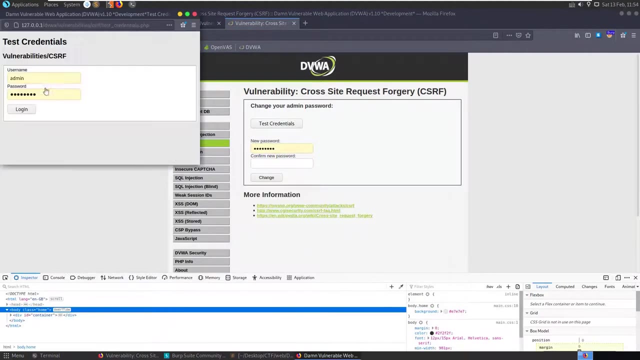 domain is the same, that's fine, and the response that we got back from that was a password changed. so now if we change our difficulty or security level back to medium, go back to our csrf page and we'll go to test credentials and then we're testing the password. here we can see that's the wrong password because we 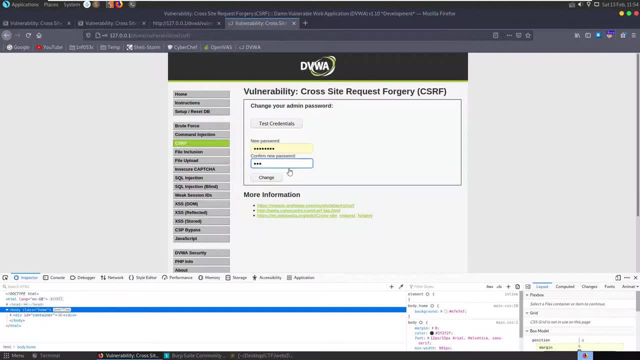 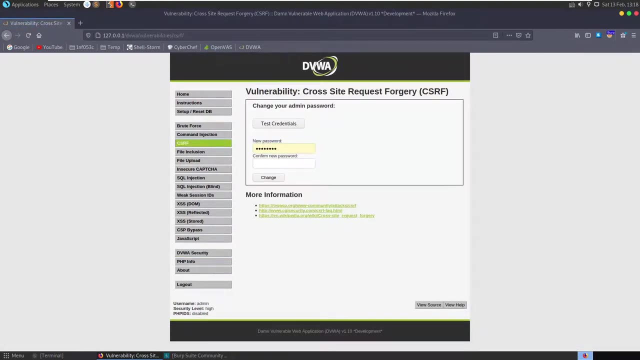 successfully changed it to test one, two, three. so let's change it back to what it should be: password, close down some of these windows and let's take a look at the high difficulty level. one thing i forgot to mention there was that the burp suite has an option if you have the 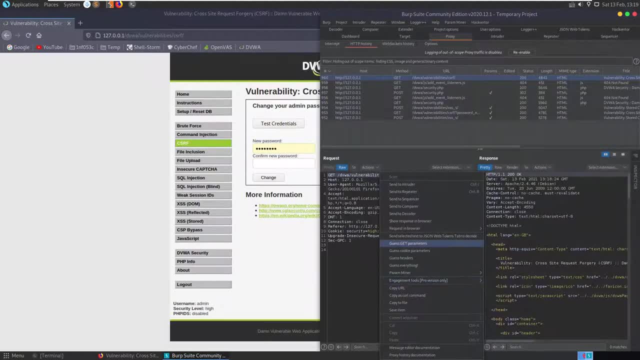 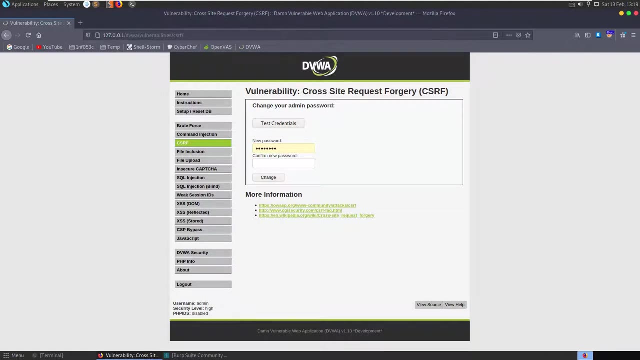 pro version, you can use the burp suite to test the password. so if you have the burp suite, you can use this. in the engagement tools, you can right click on a request or on a url and select the option to generate a csrf poc. so, um, if we wanted, if we had a form which we want to test out, csrf, csrf. 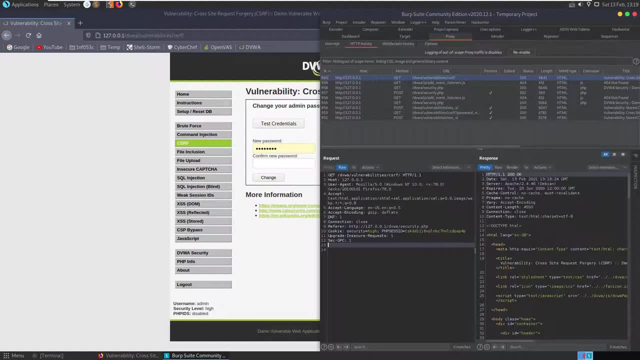 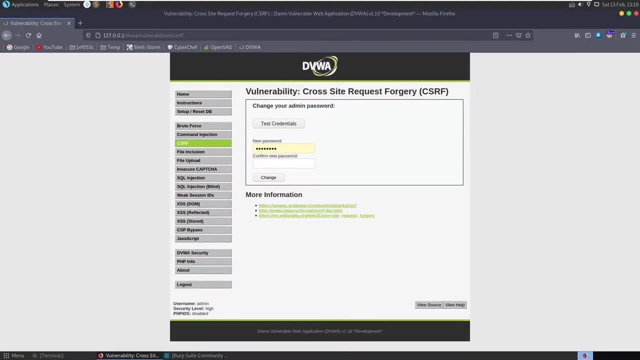 on. we could. we could automatically generate a um. we could automate the generation of a new form rather than creating that manually. unfortunately i don't have burp suite pro. i would recommend, if you're going through the burp suite academy challenges, see if you can get a trial to go through it. i did have a trial at the time and 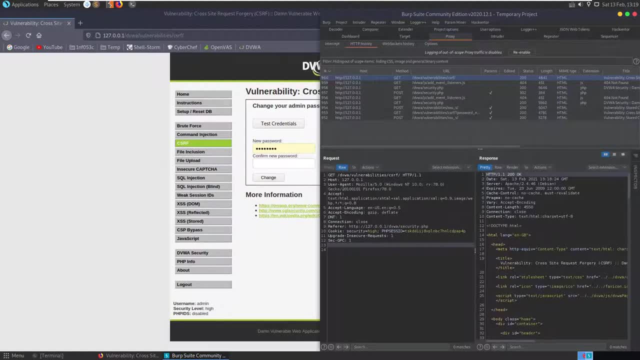 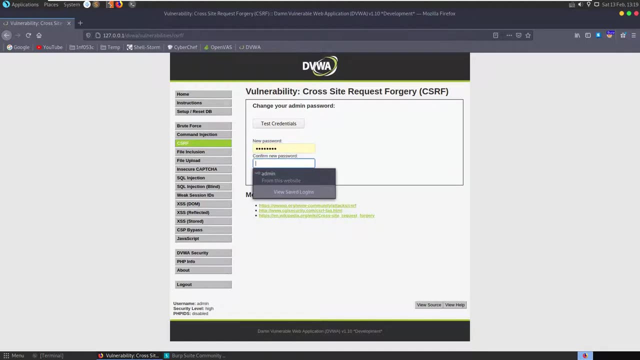 it means you can use the burp collaborator and things like that. um, but it's quite expensive. i don't have a copy at the moment. maybe if i was doing some more bug bounties and things it would be. it would, it would be worth it. but, um, okay, just gonna start by just changing the password here. 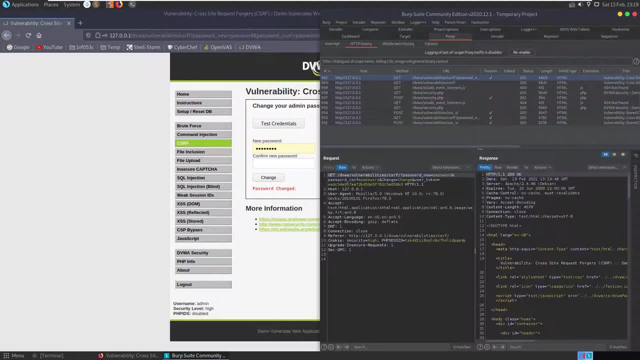 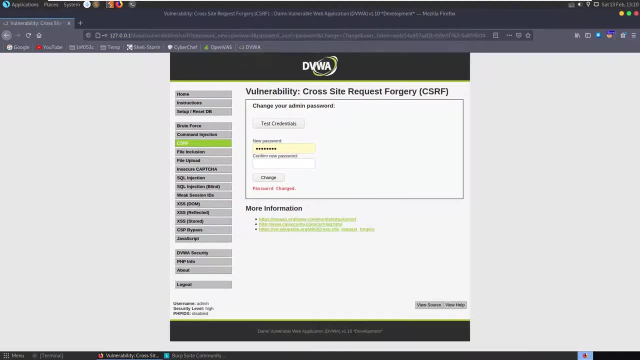 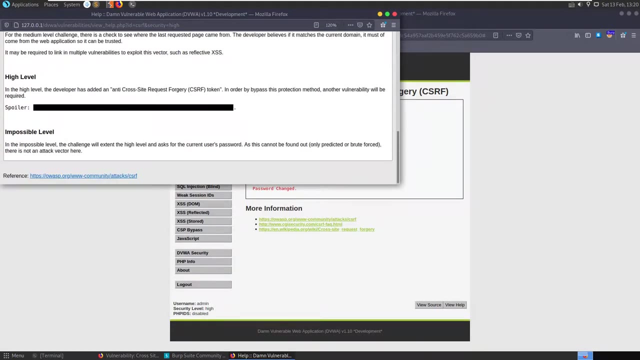 let's see what happens. we can see here that the request has gone through. it changed the password to password, which it was already anyway, and we now have this user token, the csrf. so let's um check the help. you can see here that, yep, anti-csrf token has been added in order to 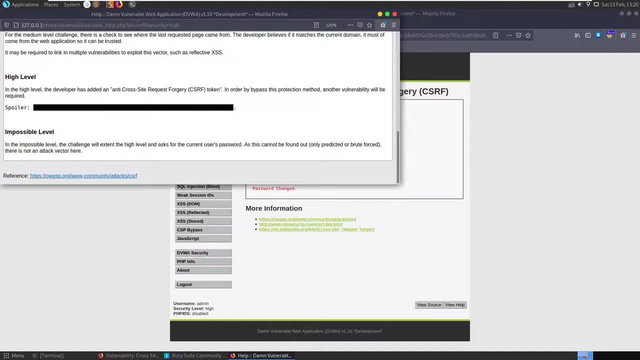 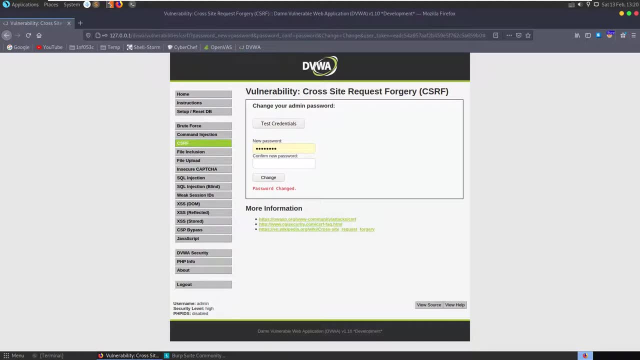 bypass this protection, another vulnerability will be required. so, um, if we, if we remember in the last set session session, if we go to our xss stored and put in our name, let's do that. and then our message: we used an image source, we said image source is equal to, and then 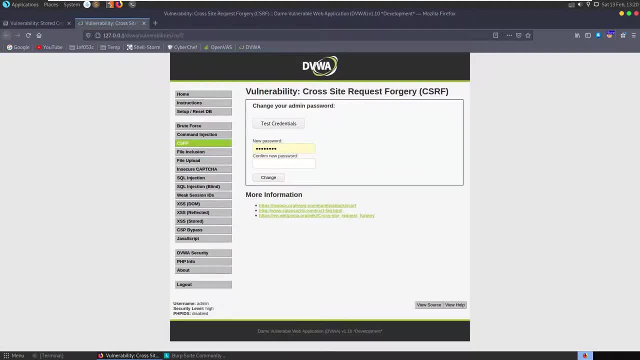 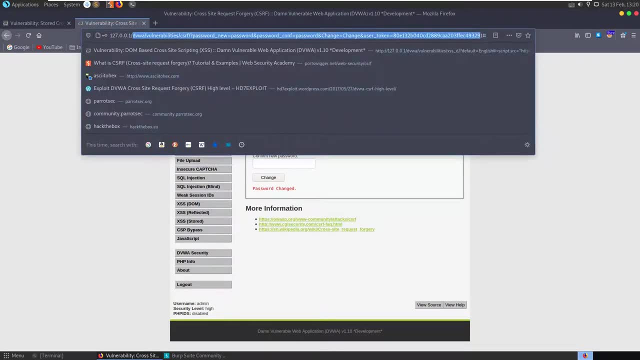 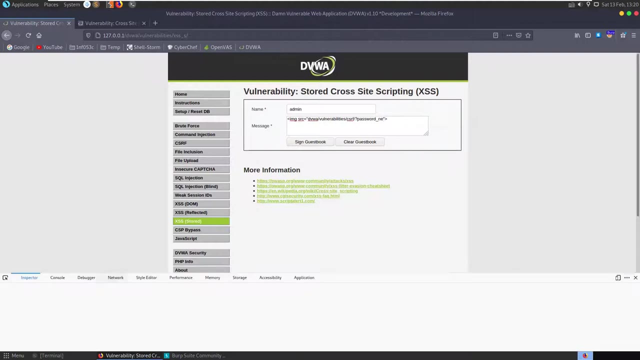 we pass in. let's grab the url, change this again, just change it to password, and we want to grab this whole thing, including the token. okay, we need to expand the size of this, so we're going to do that, and then we're going to go to our xss stored and then we're going to 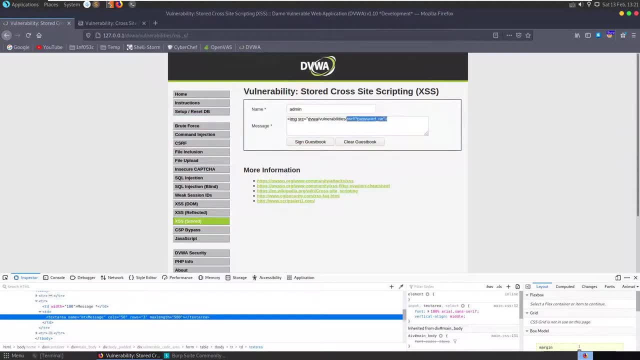 set it to whatever, set 500, and i'm going to do that again. we need a backslash first, and then that has a full token in it as well. we'll save that and then and then close, close off the tag. and if we sign, the issue is here, we get nothing back. it's not um. 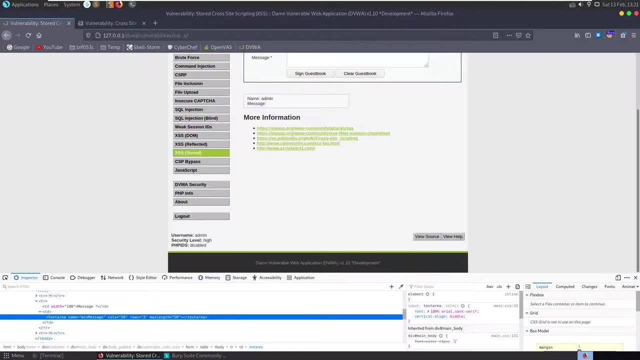 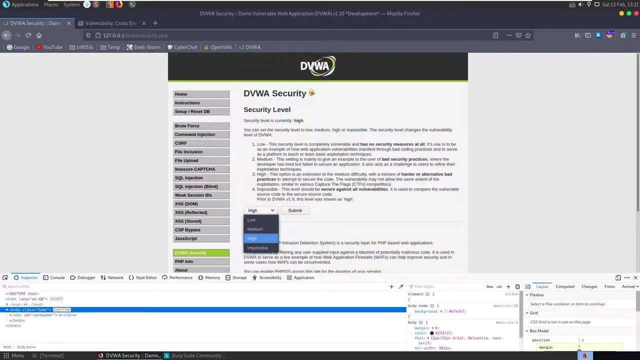 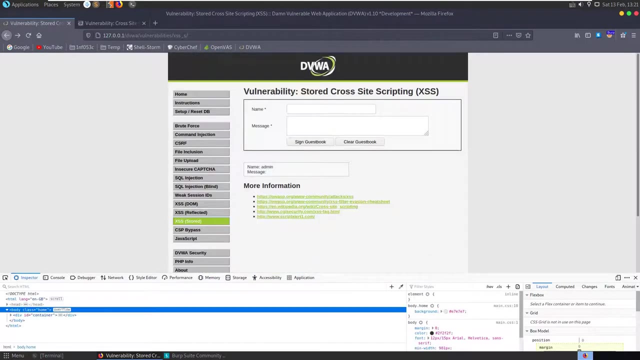 it's not actually displayed to us because we have the security level set to high. so if we go back to our security level and set the security level to medium- in fact just before i do that security level on high- ideally what we'd be looking to do here is we'd be we'd be doing okay. it's really annoying that. 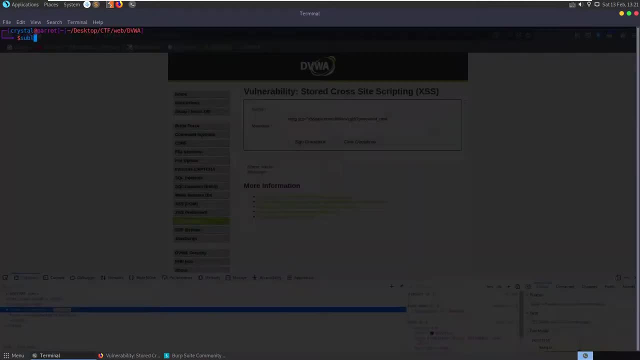 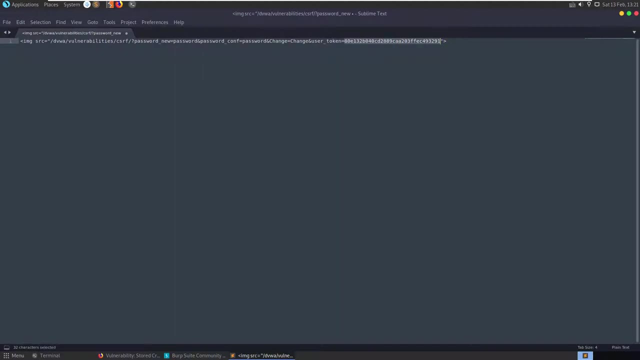 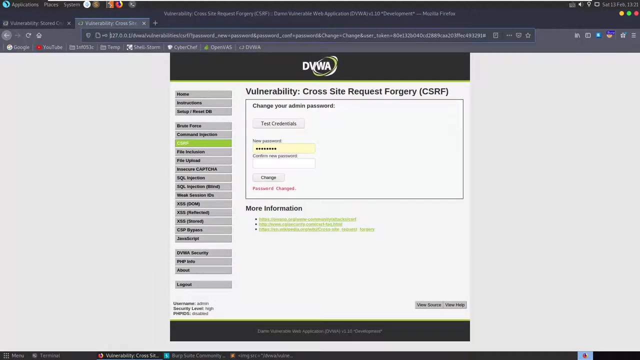 the size of that. let me paste this into sublime, okay. so ideally, what we'd be looking to do here is, instead of sending this user token, we would say: user token is equal to, and, then plus, and then, if we go in here and go to our csrf, 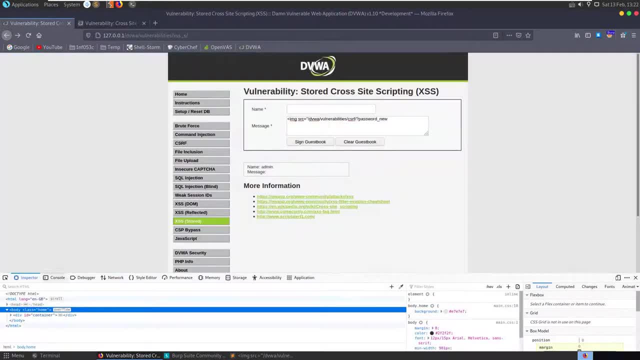 we can see that or even we'll do right here. we'll do our console and we'll say consolelog document dot. get element by name and we know that the name is user token. we can double check that. we can go to the source or inspect element. but we'll see. 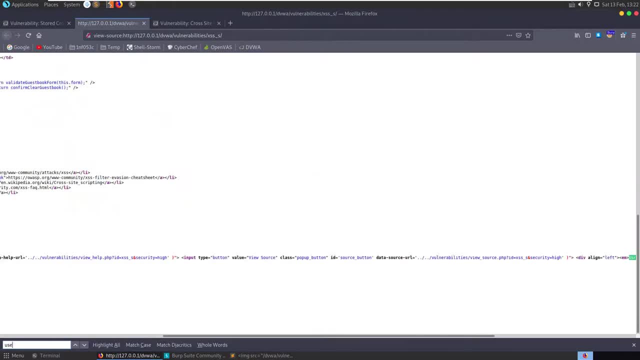 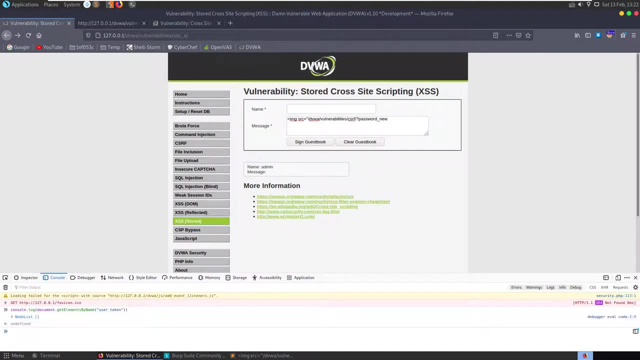 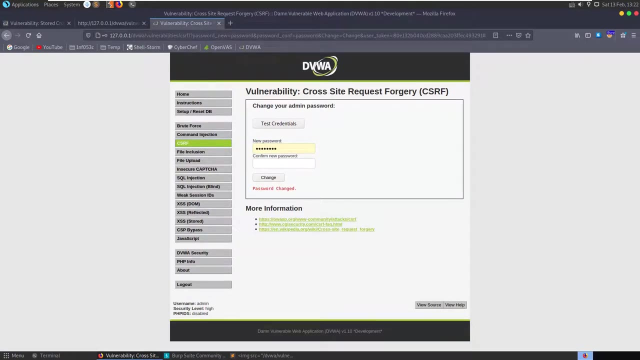 there is a user token and we can double check that and we can go to the source and we can go to the user token on this page. so let's okay. yeah, so there's no nodes on this page. let's go back to our um cross-site request forgery page. so this is on high. um, let's do the same thing. console. 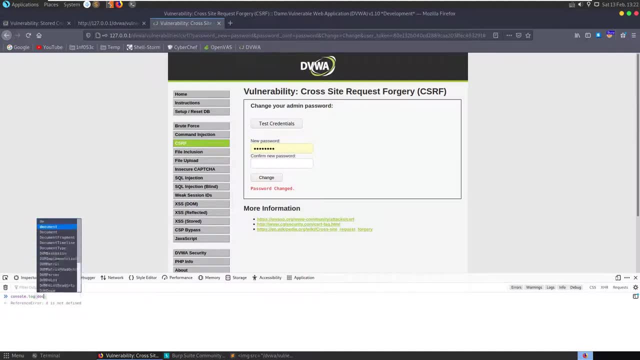 dot. log document. dot. get element by name, we give it a user token and it gets back a list of ones. so let's check out the first element and see here we've got our token, which, if we view the source, our tokens right here and it's going to change each time we refresh the page. 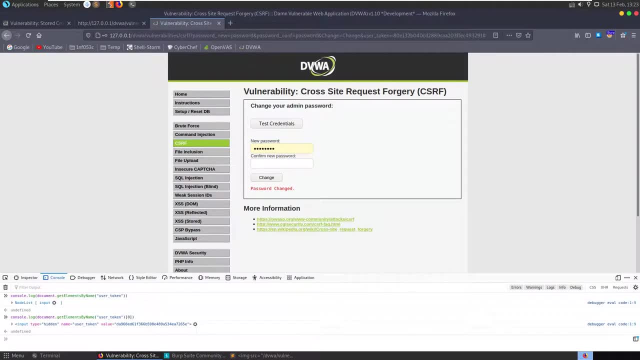 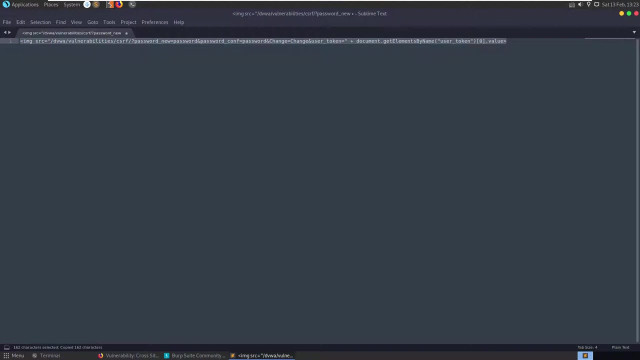 so we could be essentially saying: well, we want to do that and then grab the value of the token and it's going to print out this value each time we do that. so if we were able to just grab this and send that to the user, then it would be sending off this token as well for them, the problem. 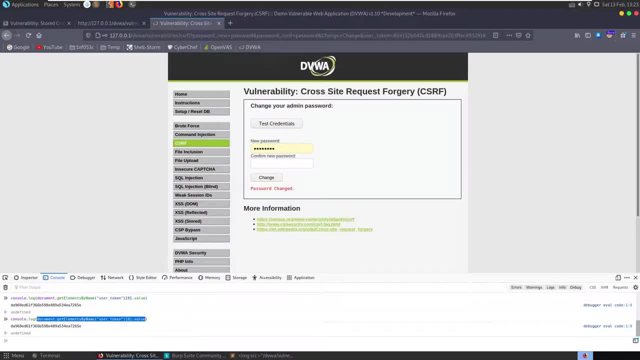 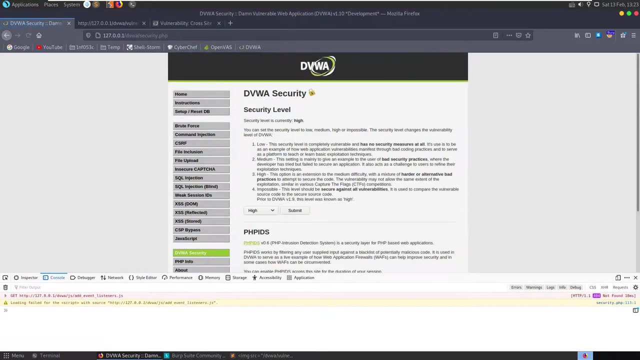 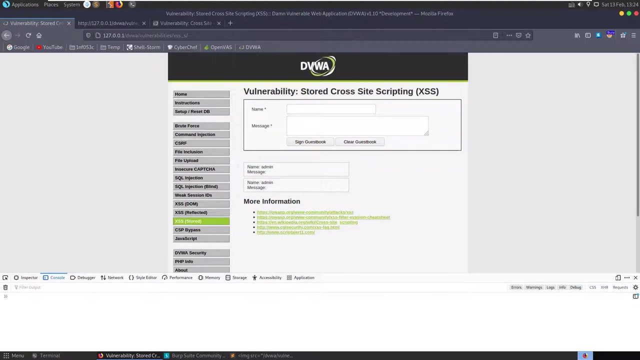 is, as we kind of saw there, that the xss stored doesn't actually take that. now if we go in because it doesn't have the, it doesn't have the csrf token there. if we go to set this to impossible, go back and submit now. go to our xss stored. we'll now see, if we check the source here, that we have the user token. 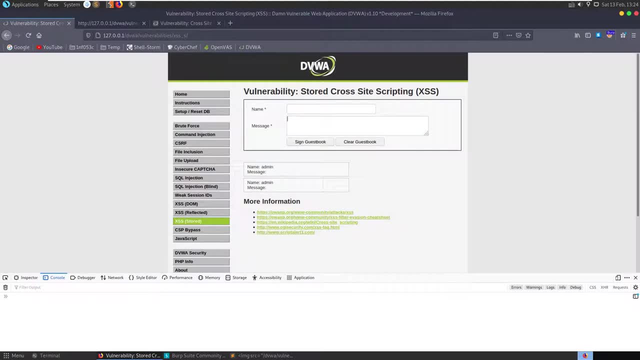 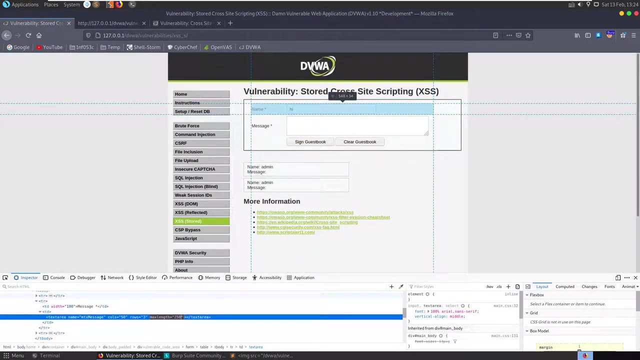 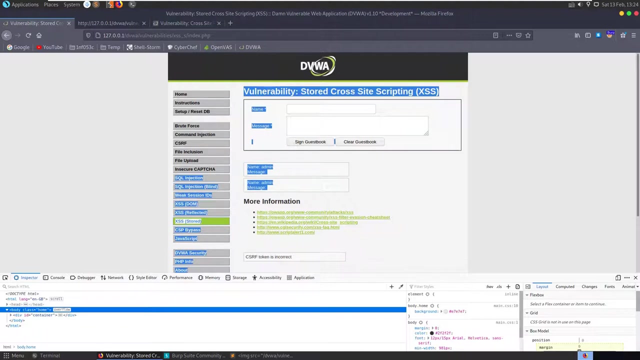 but the problem is now that it's impossible. there's no way for us to inject our, our script. so if i put in here: hi, we expand our max length and and submit that, you'll see that it doesn't even submit our request. oh, we got. their csrf token is incorrect. 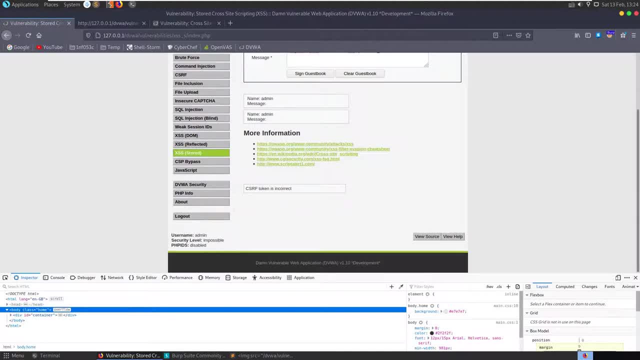 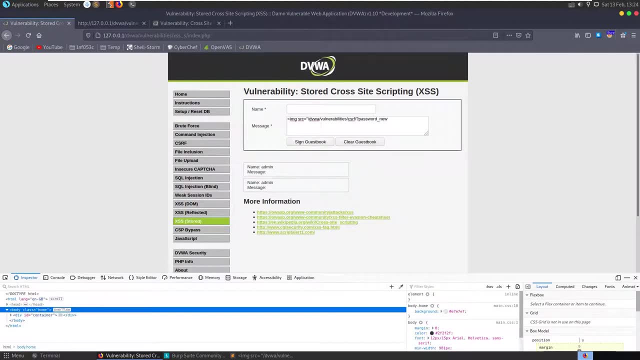 oh, so we need to actually send off the csrf token with this request as well, and but so that's the. that's the issue in terms of trying to get this done. obviously, the solution really here- okay, this is the solution- and then the login switch, and then the subscription switch, and then the login switch, and then the security work. 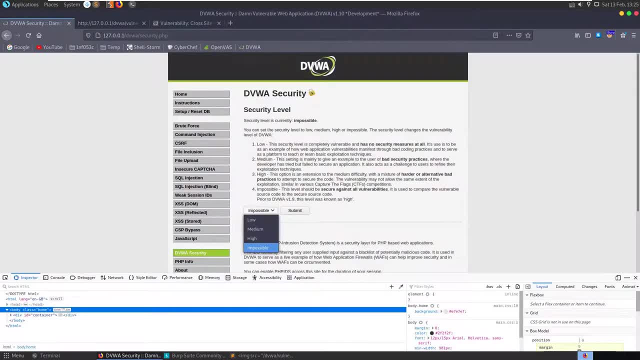 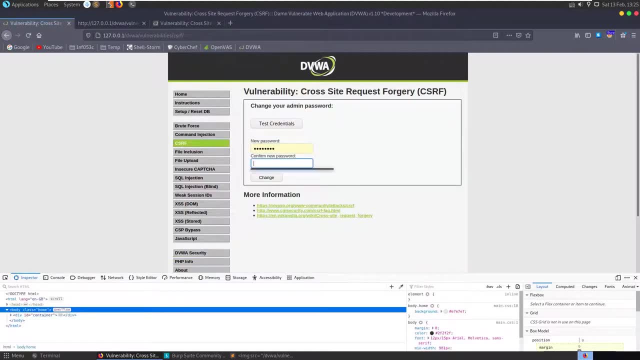 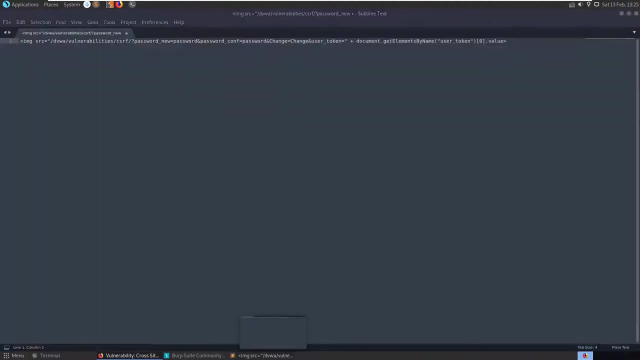 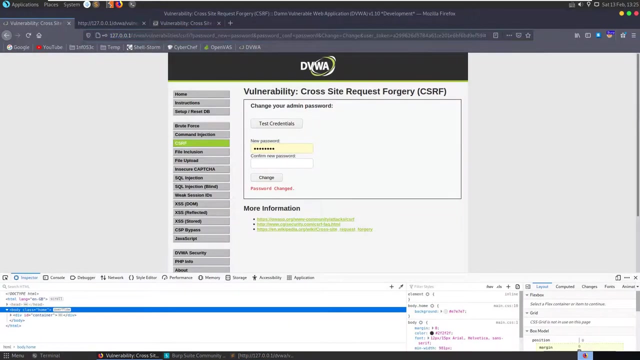 okay, this is set to impossible. let's go and set it back to high. and the solution here obviously would be to: let's change password to password. uh, grab this url. and if we were to send this url to a victim and have their token, so if we had some xss we could. 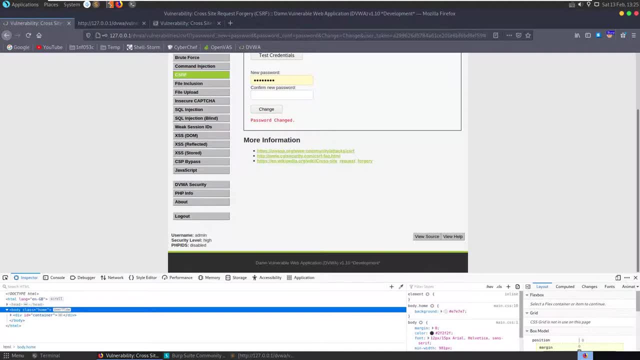 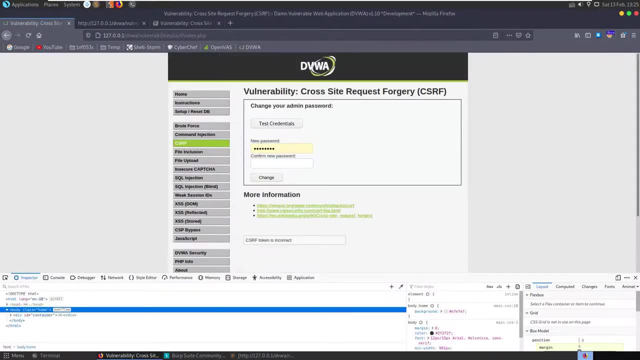 use, or we'd trick them into revealing their token to us. then we could just grab their fresh token. let's refresh the page here and let's do the. let's assume that we've done some xss injection here and say: document dot, get elements by name. 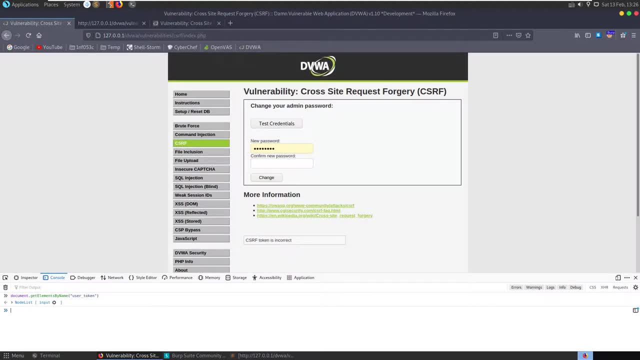 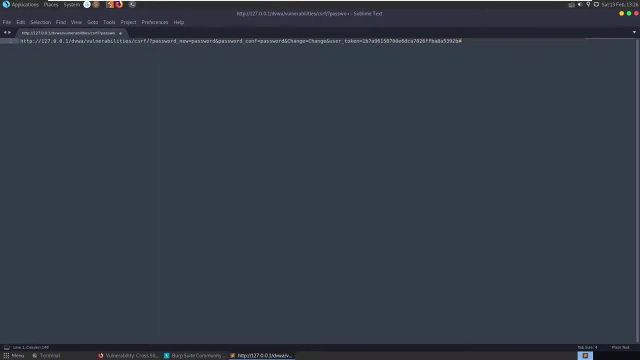 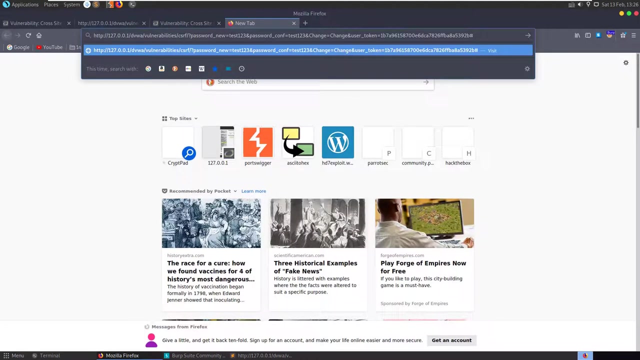 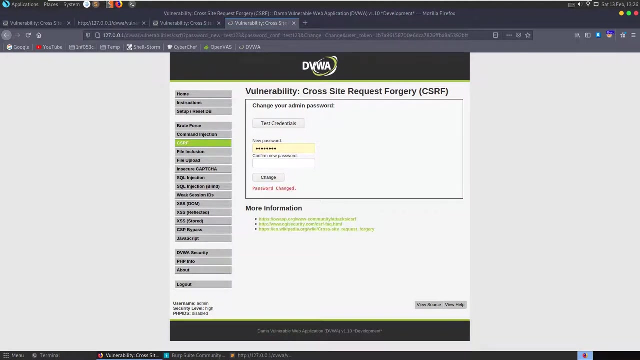 user token and let's grab our value, paste that in here and change our pass the password to test123, test123. we send this to our victim and say, hey, have you seen this cool news article? it's not dodgy at all. and then they go to the page and see this: what's this password changed? 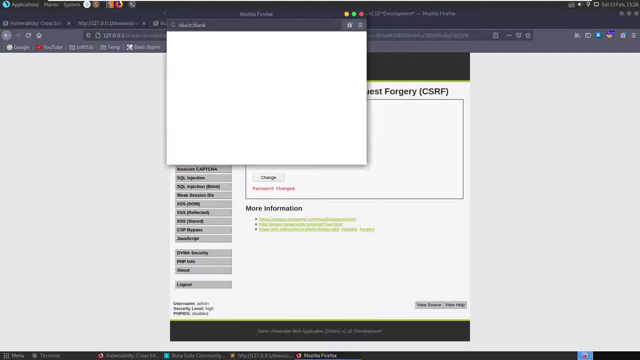 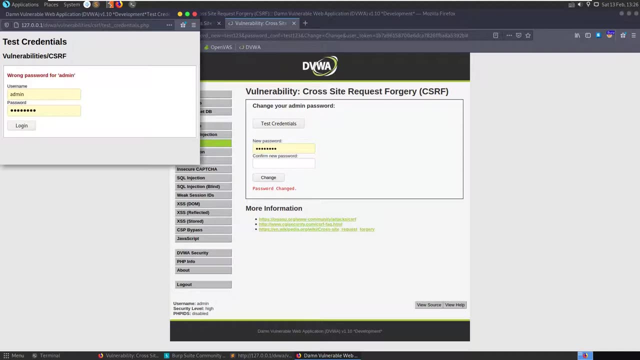 and now, if we go to test our credentials, test our credentials- we'll try to log back into our- whatever- this was facebook or something- and we'd log in with our saved credentials and we have the wrong password. so have the wrong password because we clicked on that link. but this obviously 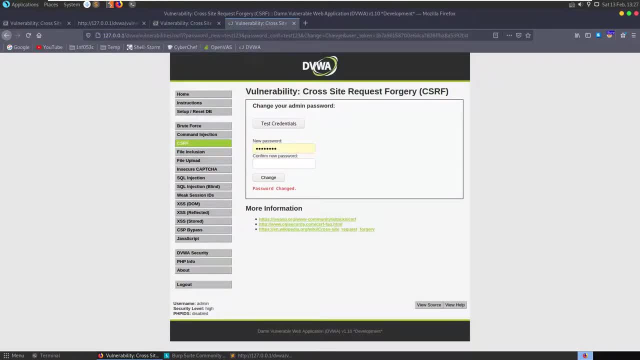 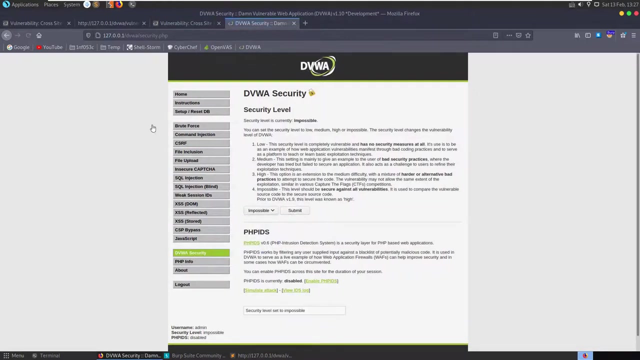 requires getting this token XSS. I mean, I'm gonna go through the XSS sections later so I guess we'll leave it at that. but we could have done it quite easily if the tokens were available on that XSS page on the same difficulty level. but yeah, let's, let's change the difficulty to impossible anyway and let's just see. 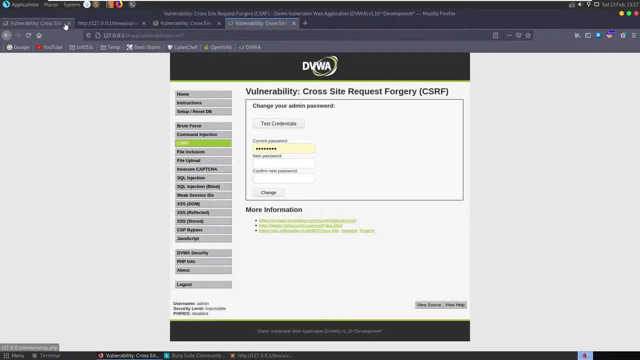 what it what we have here for the CSRF: close these down and so for impossible. we can see straight away the issue here that we need the current password in order to change the password. so if we put in, actually we need to reset our password anyway. so we'll put in our password test one, two, three, but then we 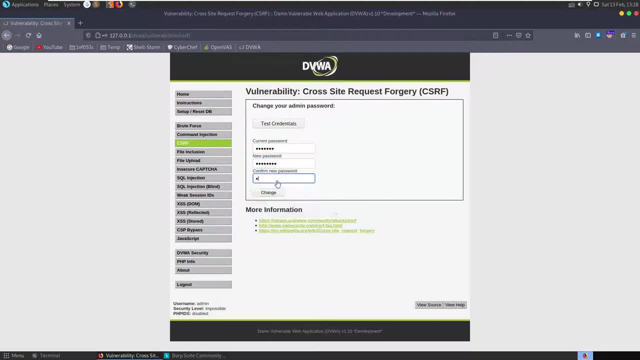 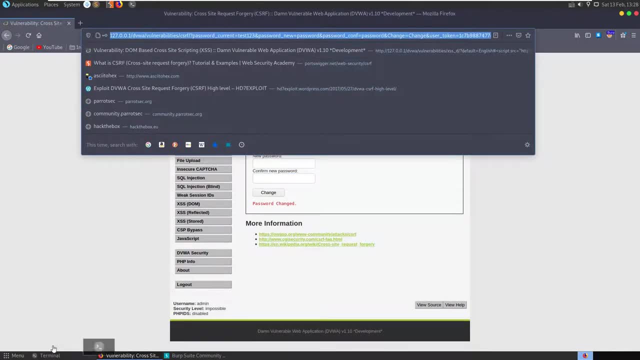 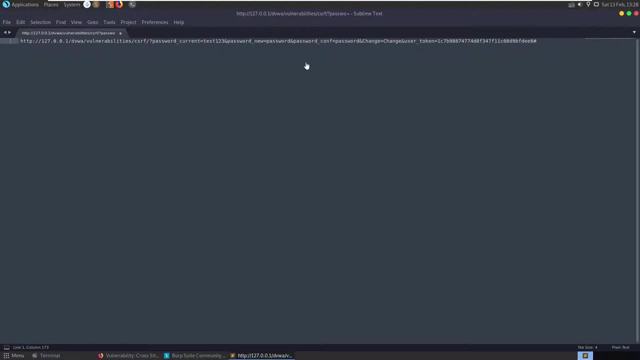 put in our new password and we confirm our new password, hit change and you can see that if we had a- let's put this in the sublime- if we had a victim and we wanted to send in this URL, we wouldn't be able to just automatically send them. 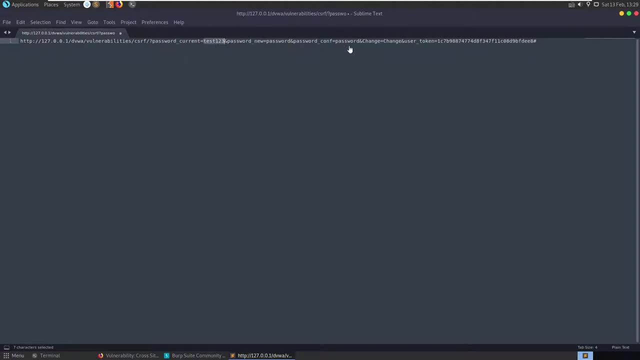 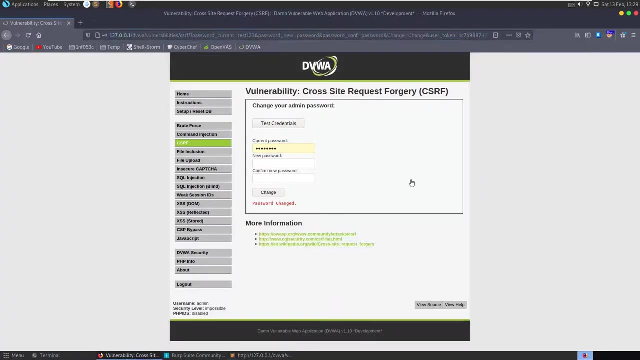 because we'd need to complete this password current. let's try and send that again now that we've changed, and we also need the user token as well. but let's even assume that we have the user token. let's grab the user token now, the new one. 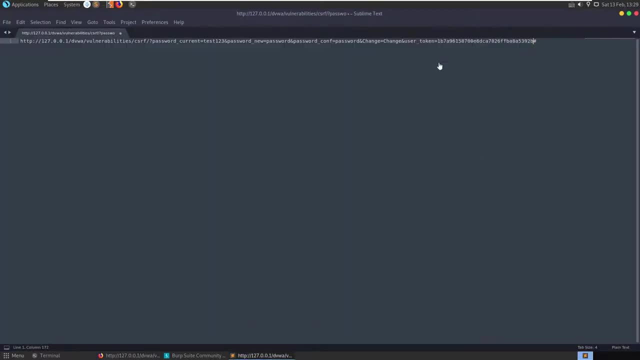 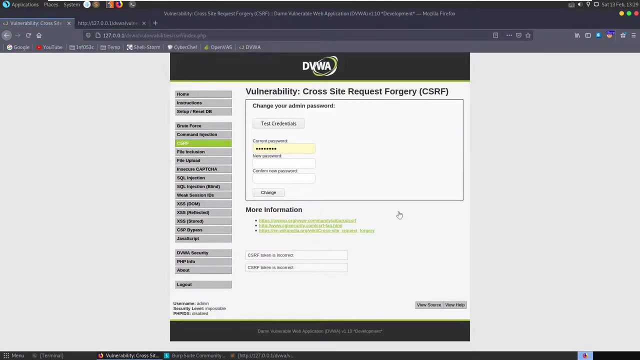 let's assume that we got this user token, which obviously is just as hard to get- well, not just as hard to get it's, but it's hard to get. but let's assume we got the user token. we didn't know the password, so we send that to the victim. they open. 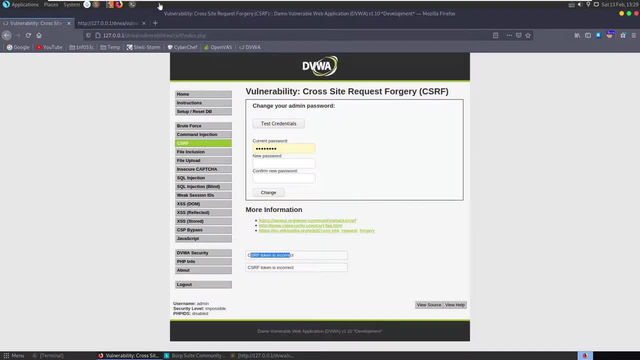 that and then CSRF token was incorrect for that one. okay, well, it would basically say that our password was incorrect anyway. and that's the, that's the impossible difficulty. let's go and double-check that and then we've got the check. see what they say here and the impossible level, the challenge will. 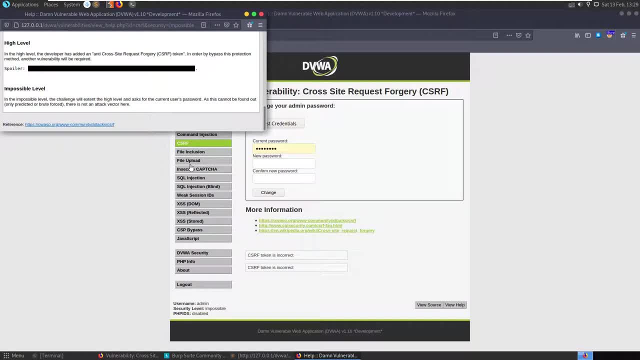 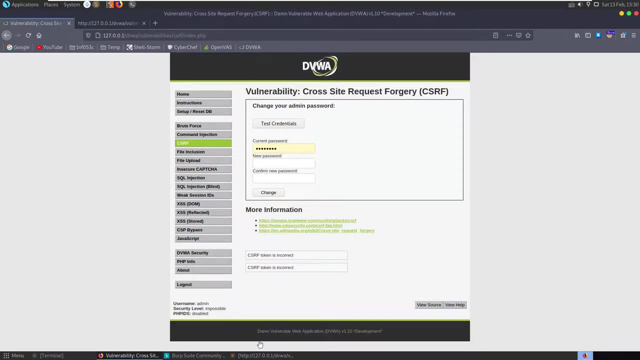 will extend the high level. extend the high level, I guess, and ask the current ask for the current users password, as this cannot be found, only predicted or brute-force. there is not an attack vector here, cool. so yeah, that's. that's the CSRF category. hope you've enjoyed this video. if anybody has any cool.